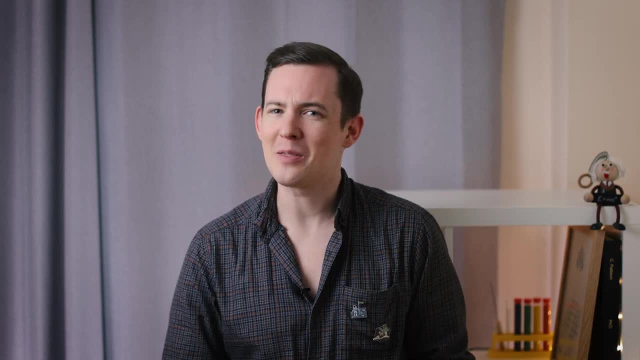 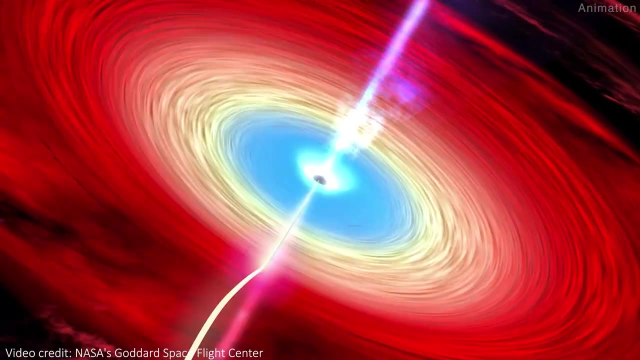 Often, when we see artists' pictures of black holes, they come with massive and powerful jets shooting out of them, seemingly blasting away from the poles of the holes. The question then is what and how, and do all black holes have them? Black holes are meant to suck things. 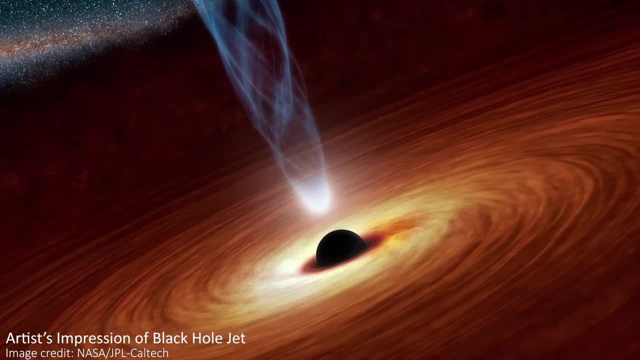 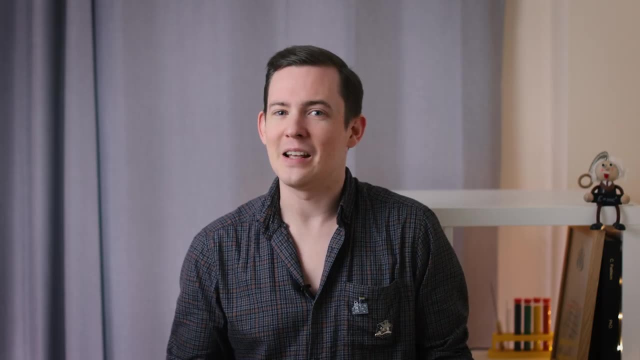 in rather than blast them out, aren't they? And why do the jets only seem to come from the poles? Why not the equator too, or any point on the surface? How does the contents of the jets even escape the huge gravitational pull of a black hole? Let's explore all. 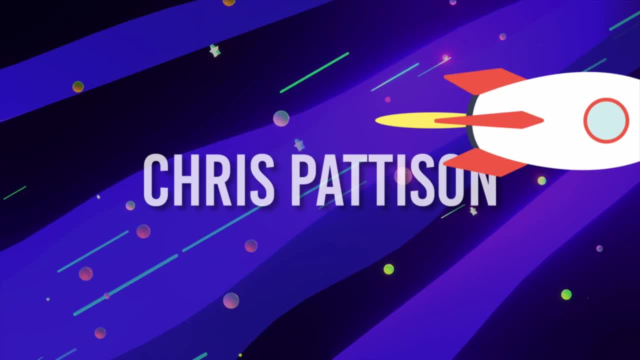 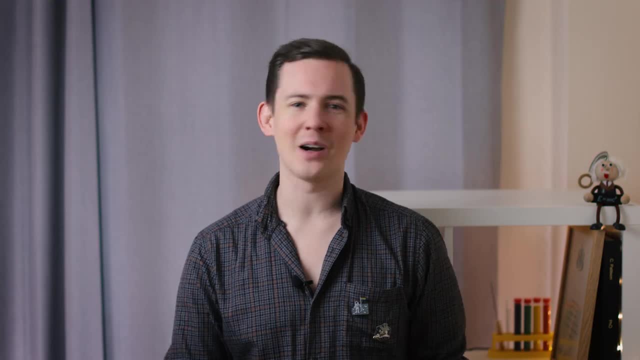 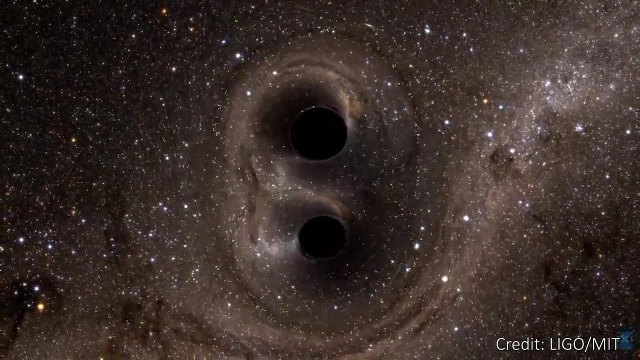 of these questions together, right here, right now. Black holes- they're the almighty gravitational object- collapse down as far as possible to create the densest objects in the universe. They are so massive and so dense that once you pass inside the event horizon of one, you can never escape. 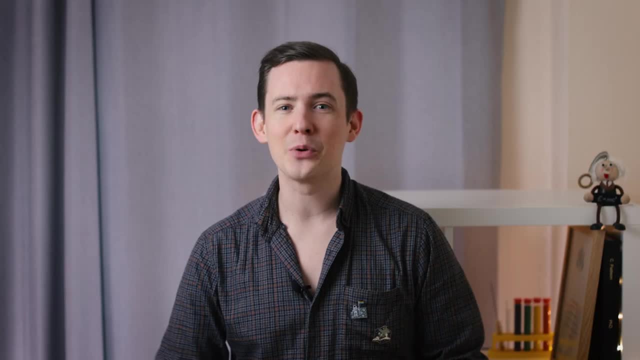 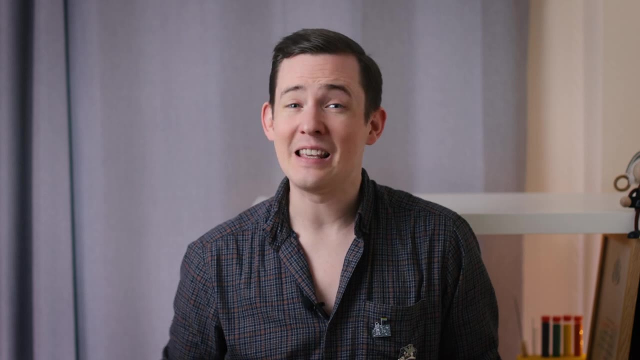 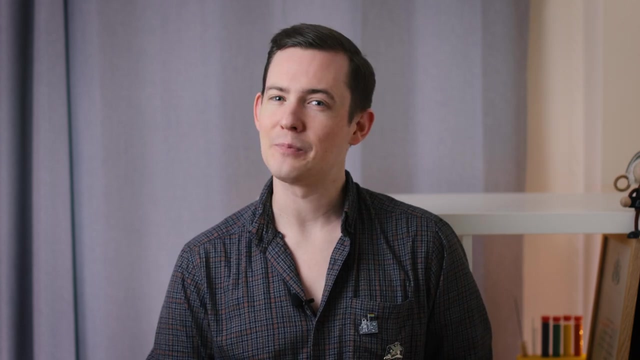 It is a one way trip. This event horizon represents the point of no return, and you'd need to travel faster than light to escape one. However, the speed of light is the absolute speed limit of the universe and it's absolutely impossible to travel faster than that speed. So, basically, 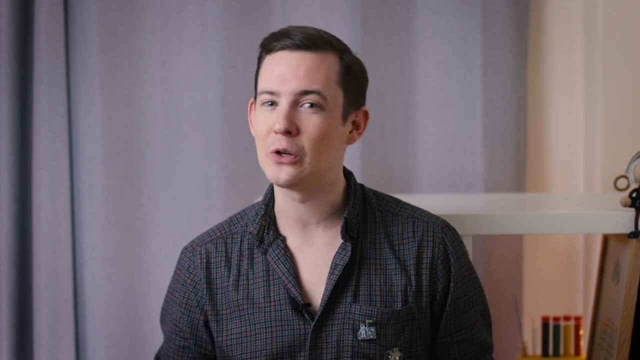 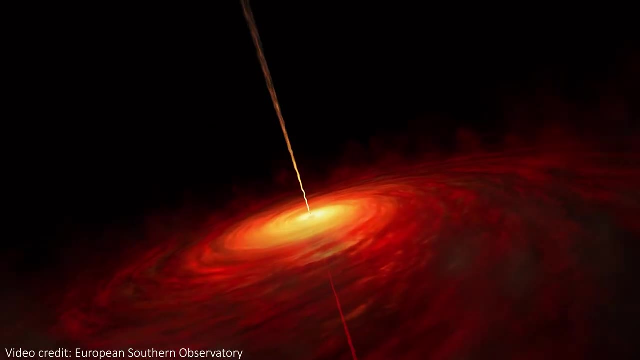 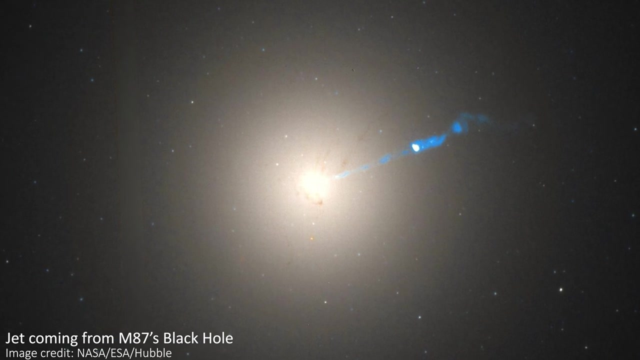 if you or anything else enters a black hole, you are absolutely forced to stay inside for the rest of time. So given all of that, it might be kind of surprising that so many illustrations of black holes seem to have these massive jets. What's more, this actually real image shows a jet. 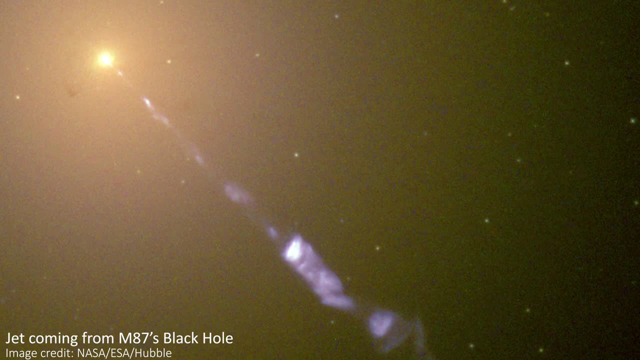 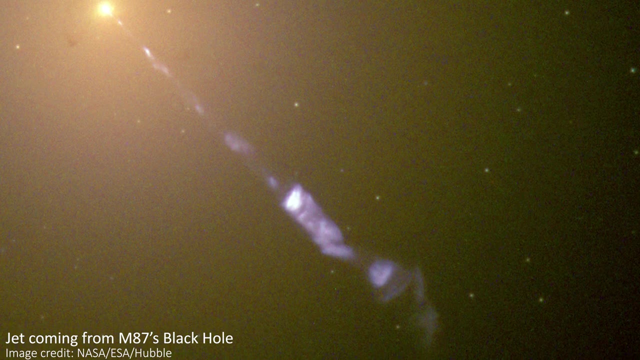 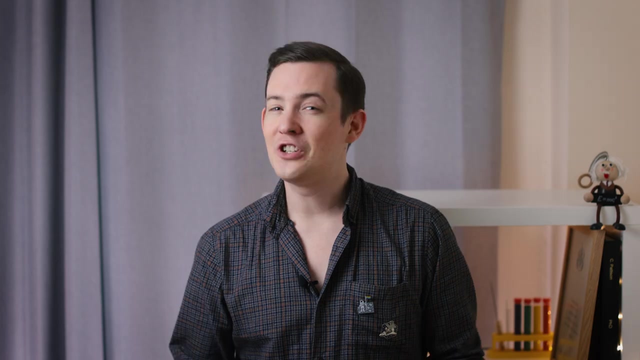 coming from a black hole too. These are Hubble images of an enormous jet coming off of the several billion solar mass black hole at the centre of a galaxy called m87. So these jets are very real and very big. This one extends over 5,000 light years from the galaxy, The. 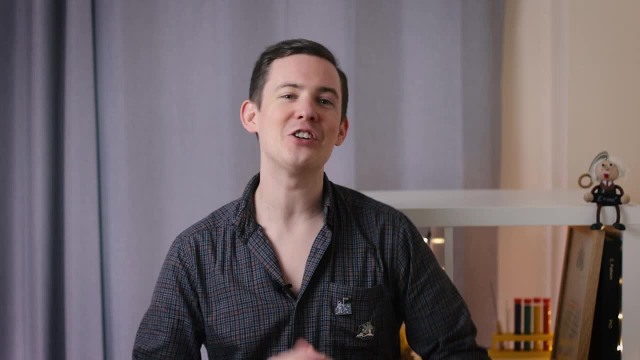 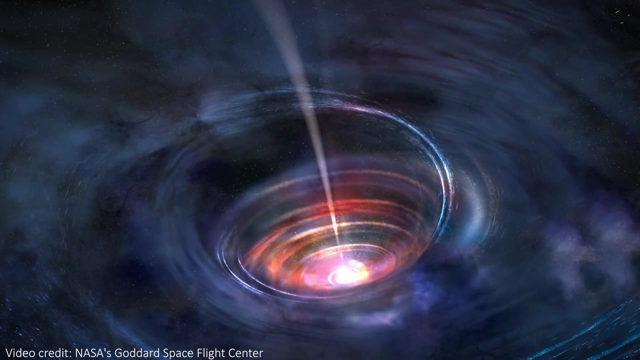 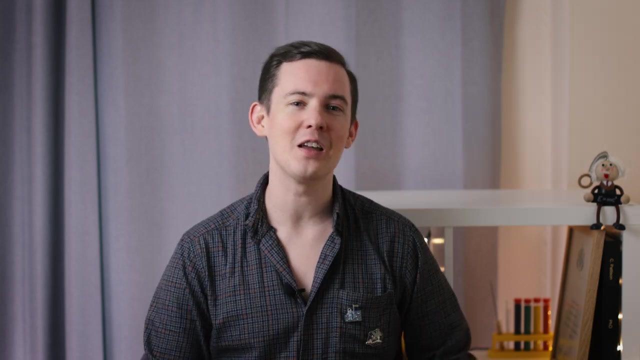 jets are usually made up of plasma, a soup of radiation and particles. Importantly, it doesn't come from inside the black hole, but rather it comes from matter swirling around the black hole that is then funnelled into these jets. Absolutely nothing in the jets comes from beyond the event horizon of the black hole. 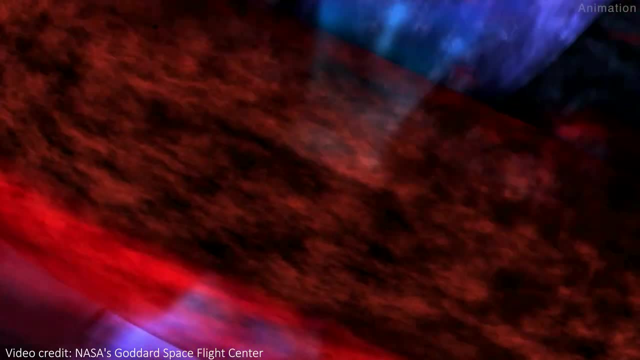 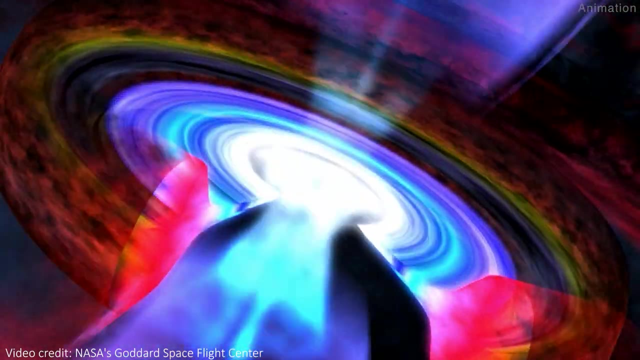 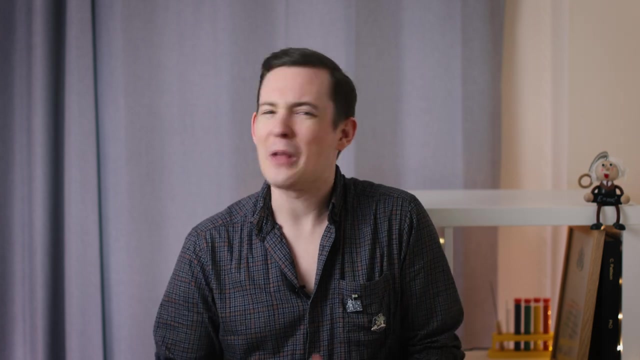 Anything in there is lost to the universe forever. This is all about black holes collecting matter around them and then the interesting physics that can turn that into a huge jet of plasma travelling close to the speed of light. Supermassive black holes are just black holes that have somehow grown to be outrageously. 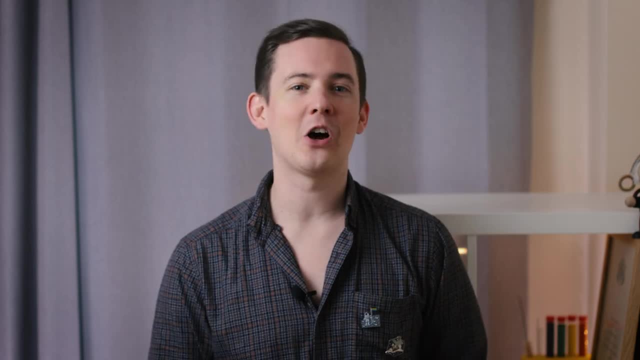 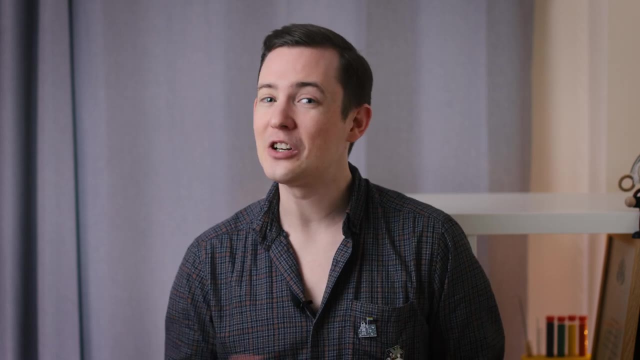 big and heavy. They are millions or even billions of times more massive than our sun and actually, as a side note, we don't really know how they get so big, and you can check out this video up here if you want to hear more about that mystery. 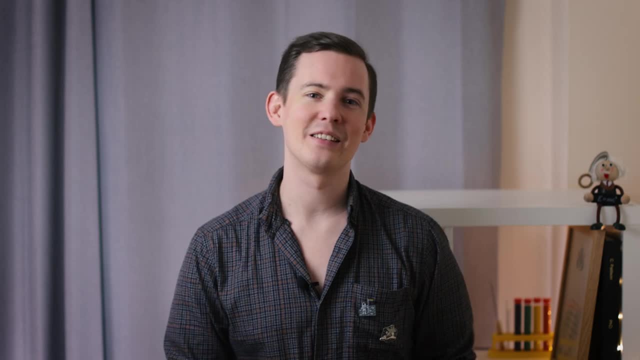 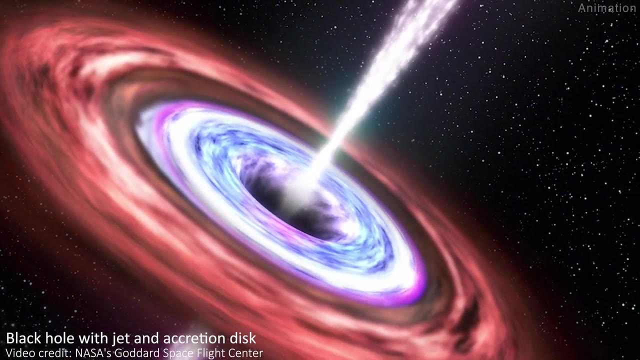 Here, though, we're just focusing on the supermassive black hole. once it exists, and in order to make a jet, you first need an accretion disk. This is a swirling disk of dust, gas and plasma. When I say radiation, by the way, I just mean light and other energetic stuff. 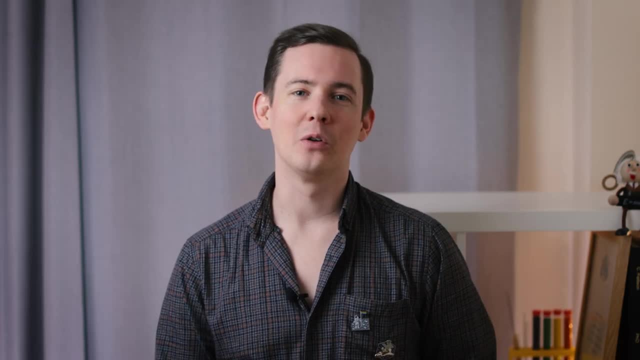 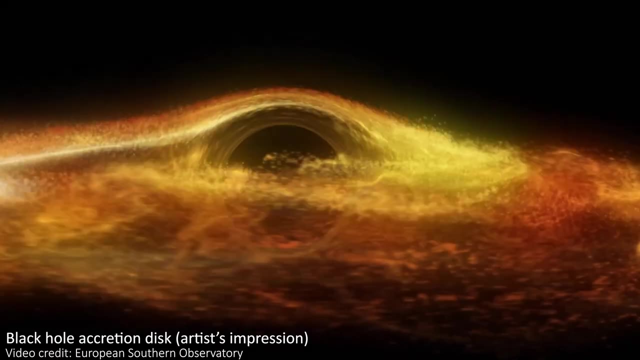 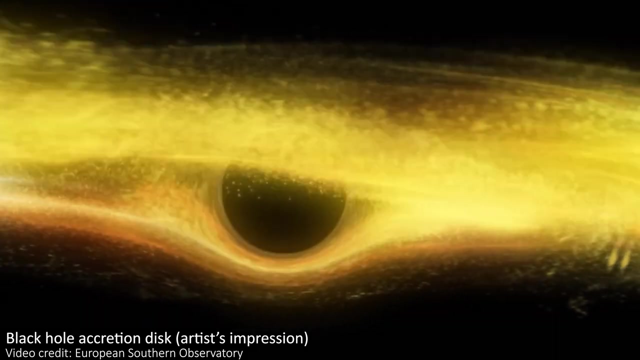 But it's mostly light. This material falls towards the black hole from all over the galaxy thanks to the huge gravitational pull of a supermassive black hole and it ends up rotating around the black hole in a pretty thin disk, That is, some of it falls into the black hole, but a lot of it gets caught up in this disk. 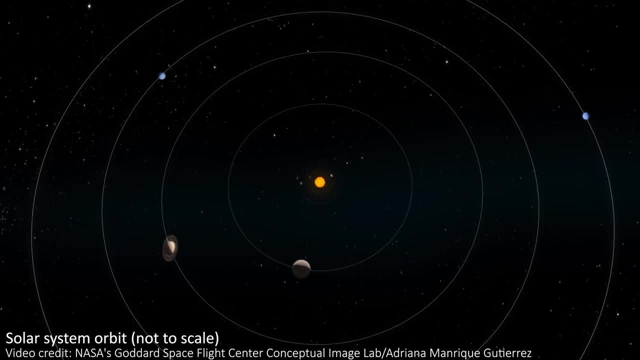 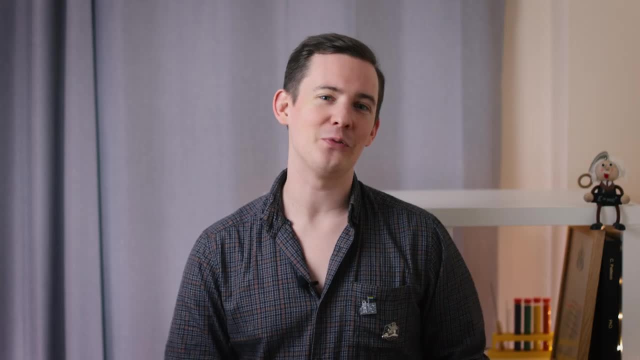 This is due to the conservation of momentum, and it's the same physics that causes our solar system to orbit in the black hole. I'll try and remember to leave some links in the description that goes into this further, so check that out if you want to explore that idea more. 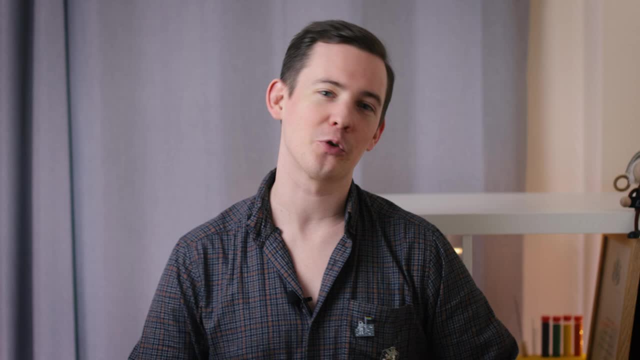 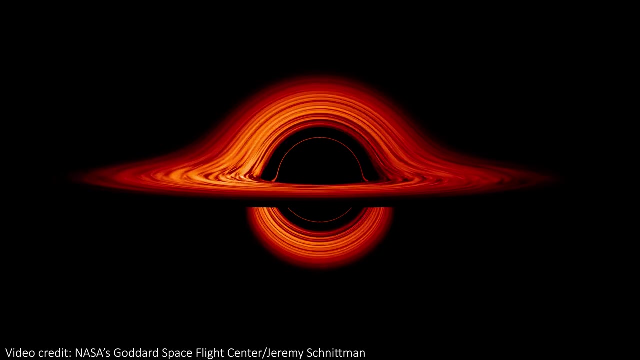 About 1 in 100 of these supermassive black holes have an accretion disk, and this is needed to form a jet. The material in the disk tends to bump into all of the other material in the same disk, and the friction of these collisions causes the matter to heat up to incredibly high temperatures. 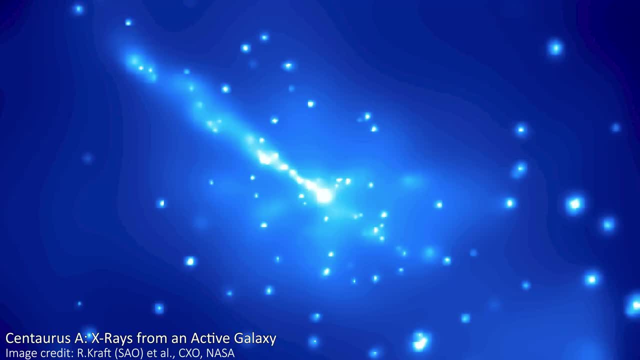 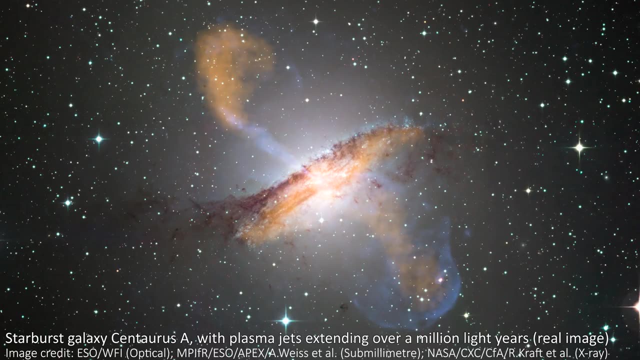 and the whole disk often starts glowing incredibly brightly. Again, It's not material from inside the black holes, but is rather material that's just near the black hole, heating up and glowing. In fact it shines really brightly, sometimes brighter than all of the other stars in the 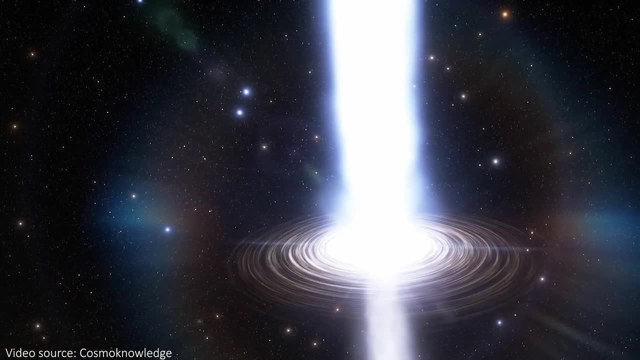 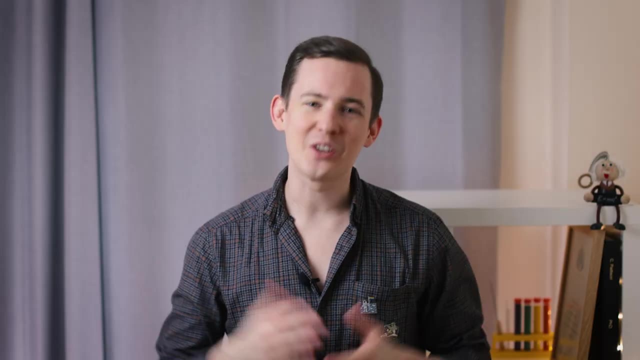 rest of the galaxy combined. These glowing disks around black holes are called active galactic nuclei, AGN or sometimes quasars. We can even see these accretion disks in direct images of regions around a black hole. This is an image from the Event Horizon Telescope. 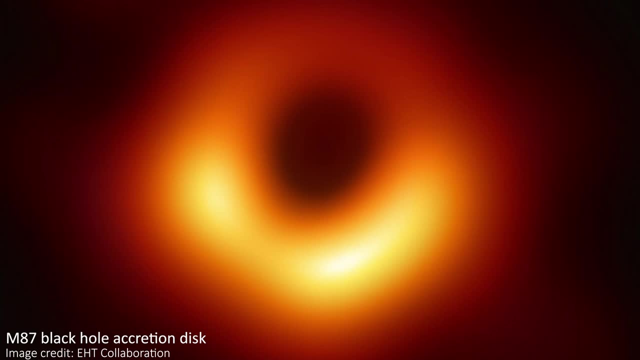 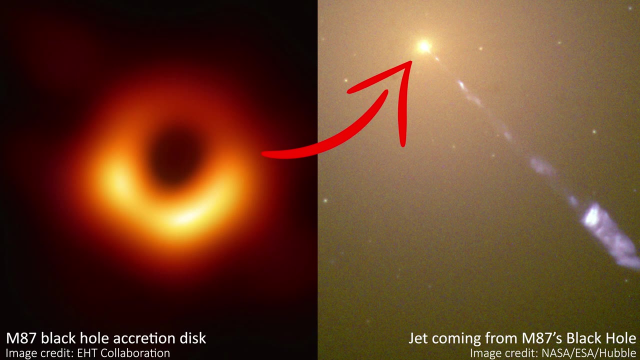 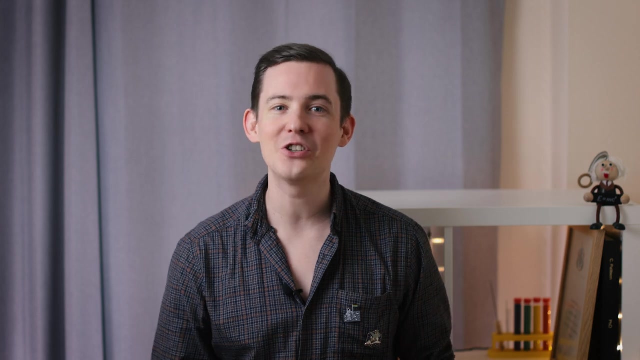 We can see the black hole in M87, whose jet we saw earlier. So we know this disk and this black hole are powering a huge jet. In fact, the brighter the disk, the more powerful the jet. The jet itself, though, is produced through a combination of the rotation of the black. 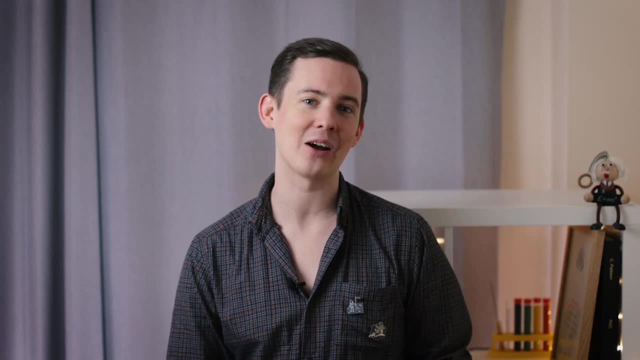 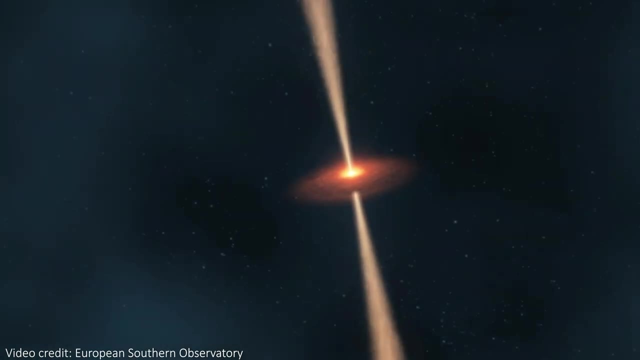 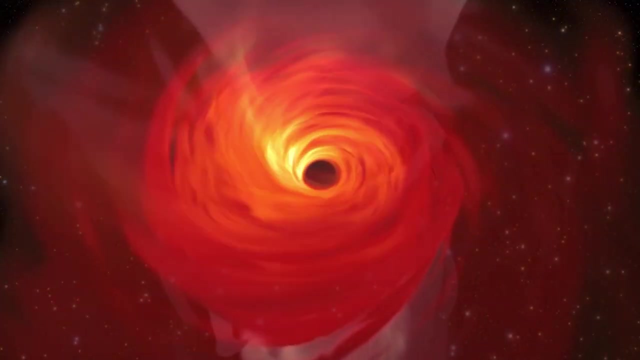 hole and its accretion disk and the magnetic field of the black hole too. The particles in the disk end up being electrically charged through all of the collisions they endure, And this produces a powerful magnetic field. A rotating black hole is a powerful thing, and the rotation actually drags the space. 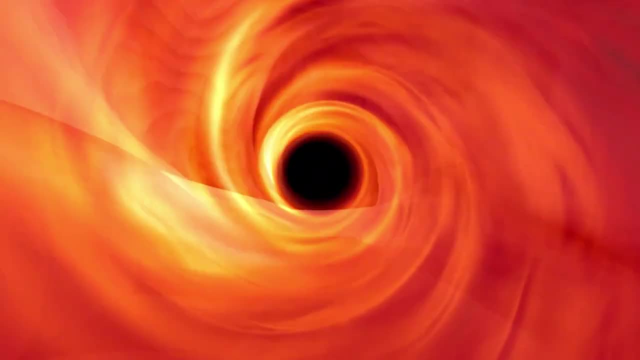 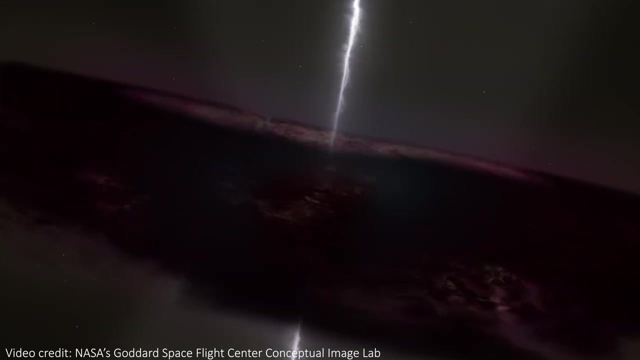 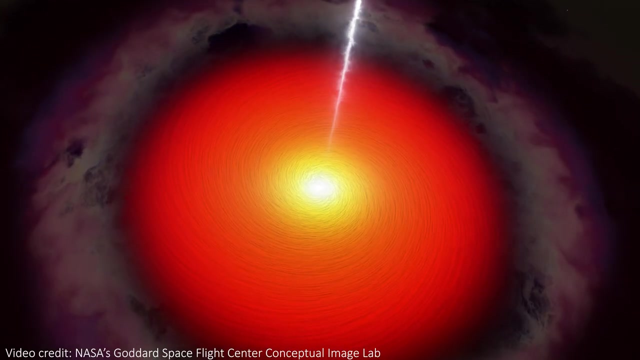 around the black hole along with it in an effect called frame dragging, But it also pulls and twists on the magnetic field too. We end up with a magnetic field that winds into a cone at the pole of the black hole. This twisted field then accelerates charged particles and radiation from the disks to 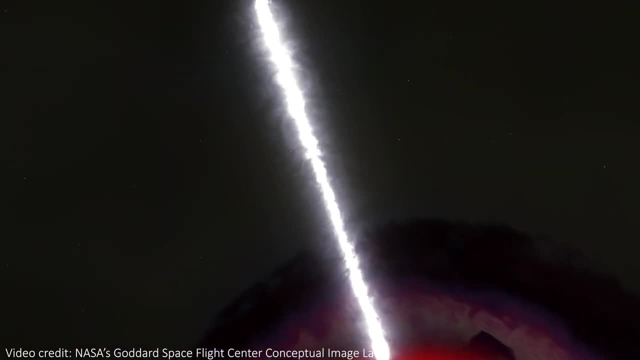 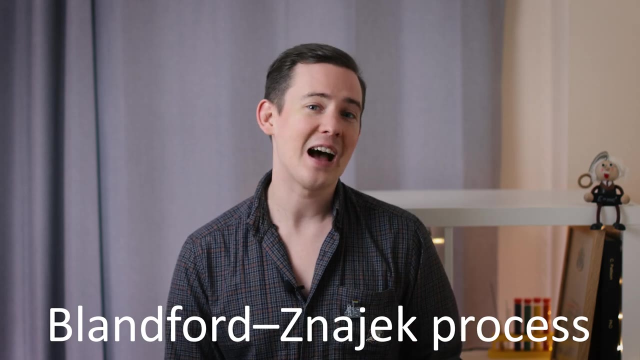 the poles, And then the black hole has to blast away in the powerful jets we're talking about here. This process is called the Blanford-Zenayak process, and it's currently the leading theory we have for how these jets are produced. 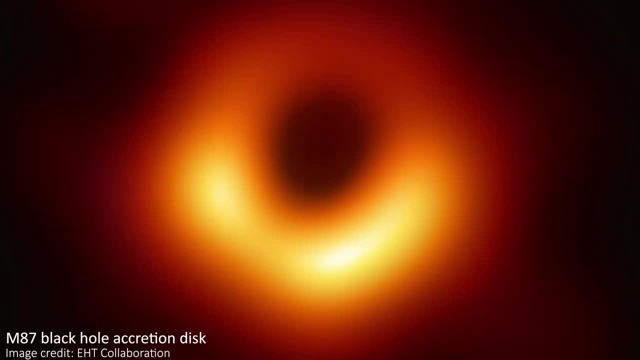 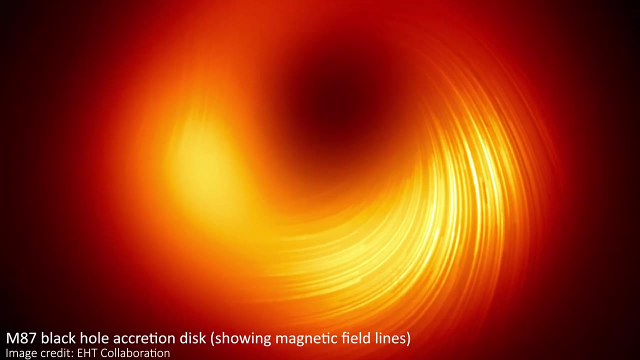 In fact, let's go back to that M87 image, and we can also see an image that shows the magnetic field of the disk too. You can hopefully start to imagine how this magnetic field and the rotation of the black hole can cause all the right conditions to start producing these jets. 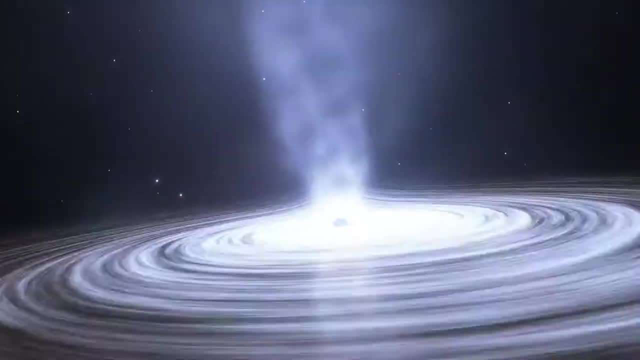 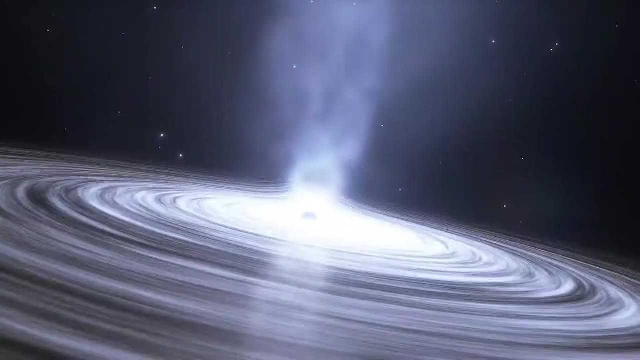 black hole somehow. So, given a long enough period of time, the rotation will slow down as it's giving up that power in order to accelerate the particles away from the black hole in the jet- And these jets are some of the most powerful things we've ever observed in the universe. 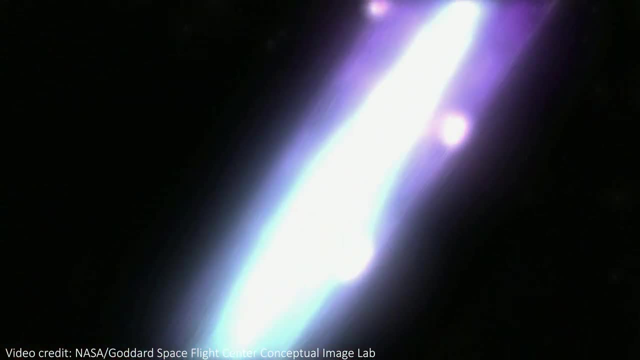 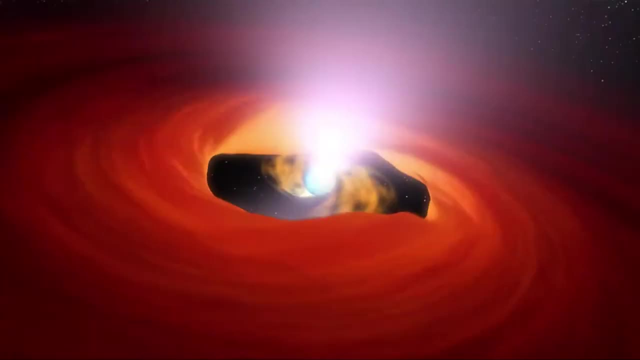 so they've got to get all of that energy from somewhere. If a jet is pointing straight at us, rather than call it a quasar or an AGN, we call it a blazar. And if the jet is processing and passing over us regularly, then we call it a pulsar. and these are amazing objects. 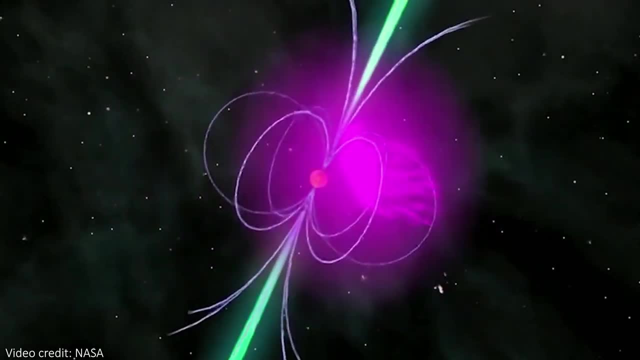 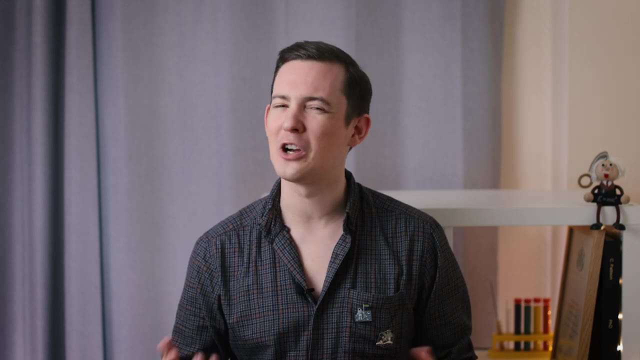 They can be used as galaxy-sized gravitational wave detectors, and they're also some of the most precise clocks in the universe, so we'll definitely be talking about them more in the future on this channel. Be sure to subscribe so you don't miss any of that excitement.